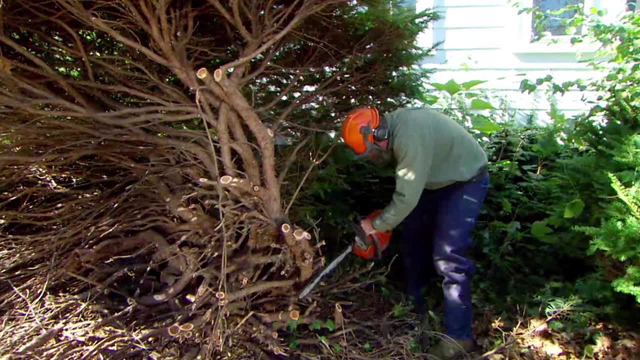 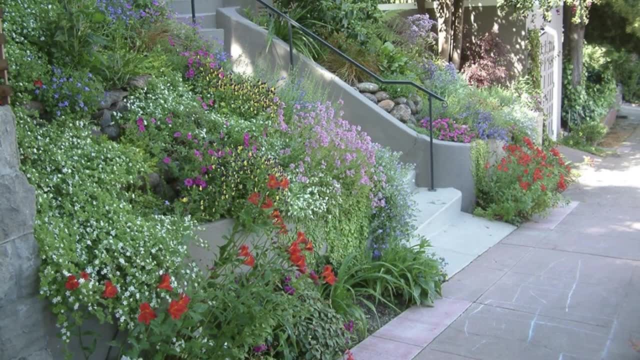 and are non-natives, so removing them and replacing with better selections can be a win-win. Transforming your garden into a fire smart and biodiverse landscape may seem like a daunting task, so make a plan to tackle it in steps to maximize your maintenance dollars. 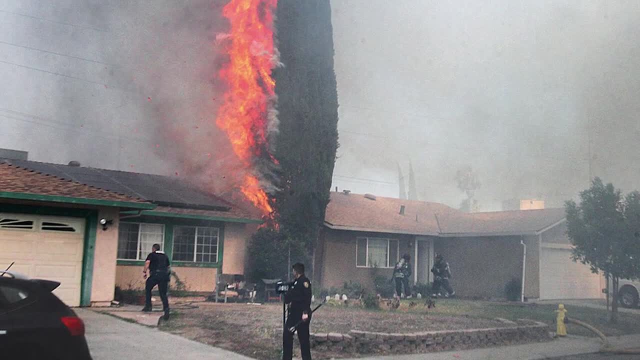 and minimize your time investment. Start with undesirable plants in the zone zero within five feet of structures. The ones that fire start with are the ones that are most likely to die. The ones that are most likely to die are the ones that are most likely to die. 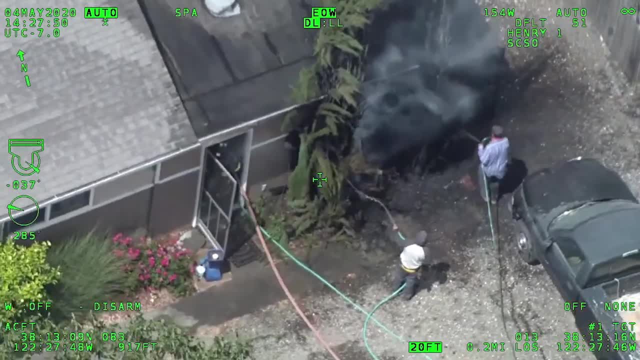 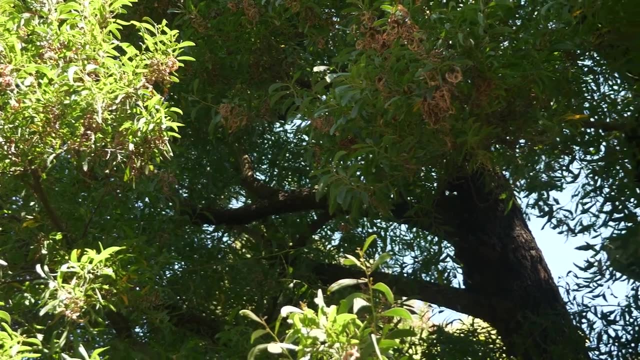 This fire-safe marine recommends being removed due to their tendency to build up dried material. An example are these black Acacia trees overhanging this garage. This invasive species has a lot of dried material in the canopy and on the ground during fire season. The benefits of 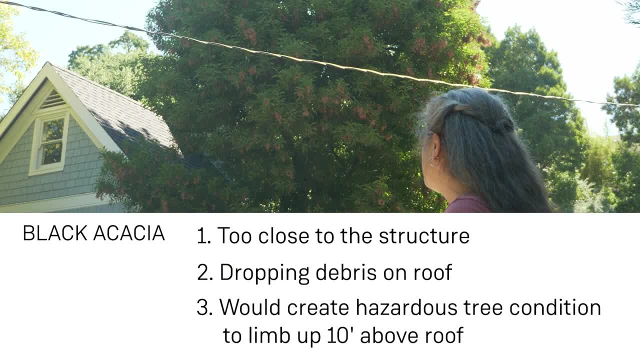 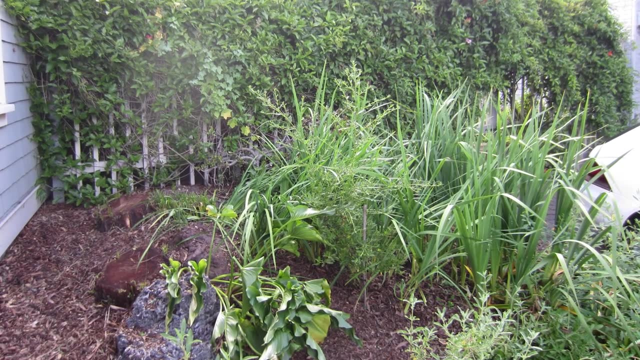 shading the garage from afternoon sun and some bird nesting activity did not justify the fire hazard and limited biodiversity they help to support. There were much better options for this location. The trees were removed and replaced with ceanothus, a native tree, and smaller natives, including salvias and. 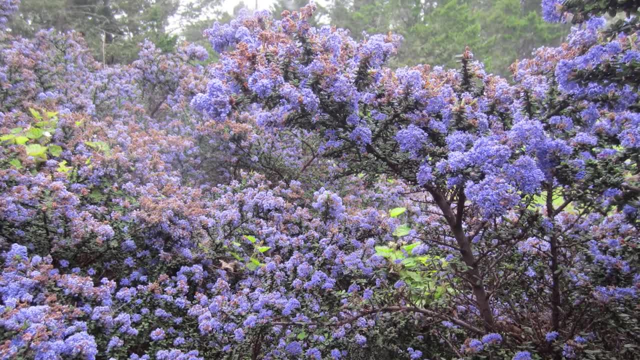 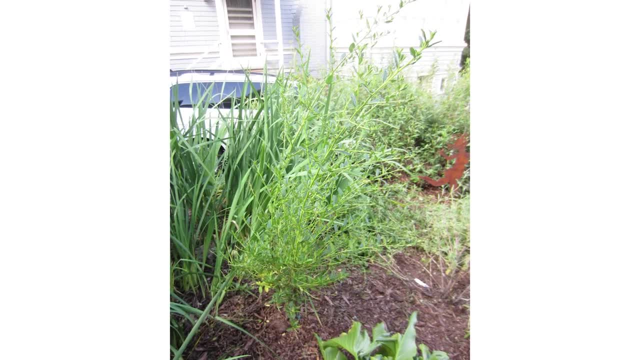 douglas iris Ceanothus is an early blooming plant that evolved with native bees and supports them with nectar and pollen after their post-winter emergence. In addition, it's relatively slow growing and can be easily kept pruned at an appropriate distance from the garage. There's 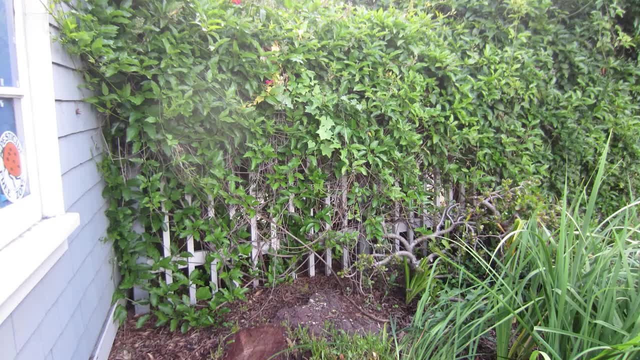 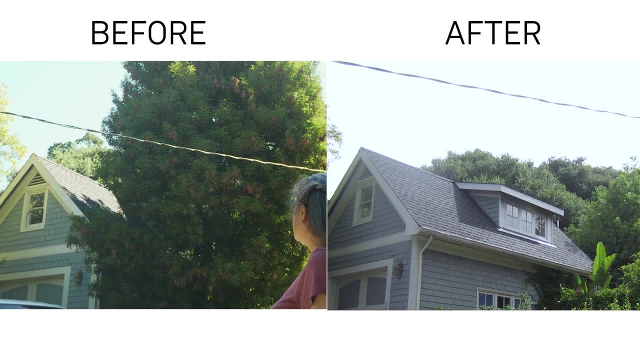 still work to do around this planting bed. The vine needs to be cut back and ideally, the fence would be replaced with a non-combustible material. But take it one step at a time and prioritize the biggest hazards to your home From a bee perspective. density of plant type. is important. Bees prefer to forage on a single plant type. on any single foraging trip, Larger patches, at least three feet by three feet when the plants are mature, will attract the most bees If you like the look of dense plantings and the beneficial insects they support you. 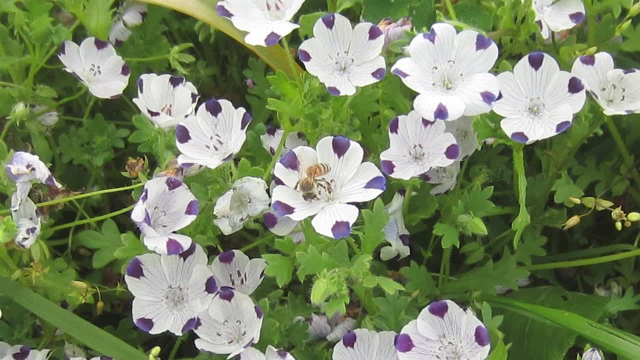 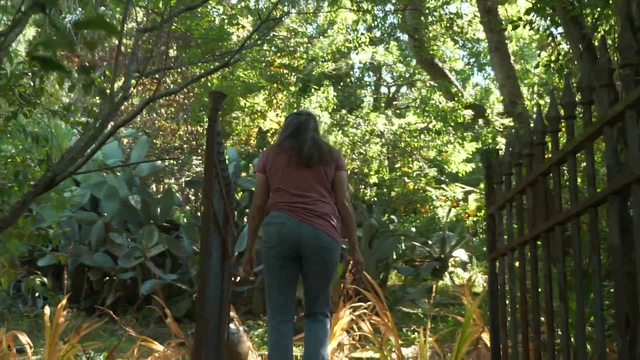 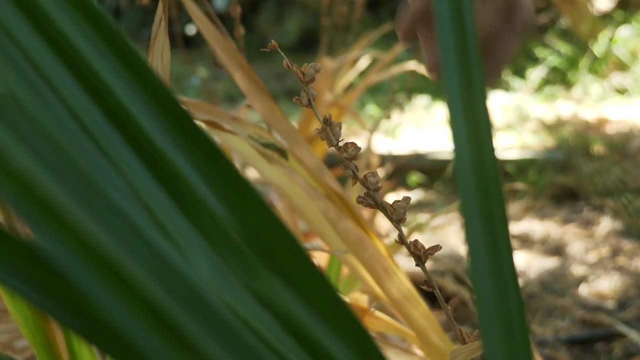 can take advantage of bees. In fact, other than ensuring dried planting material is removed by fire season, you may have to do nothing else, including watering. You can collect seeds from annual plants that you and the pollinators enjoy. It'll save money. Just collect the seeds when dry and 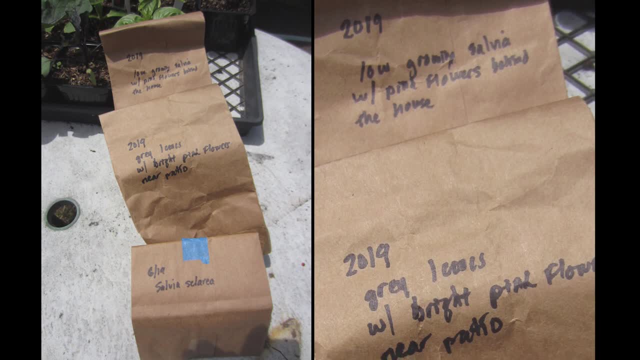 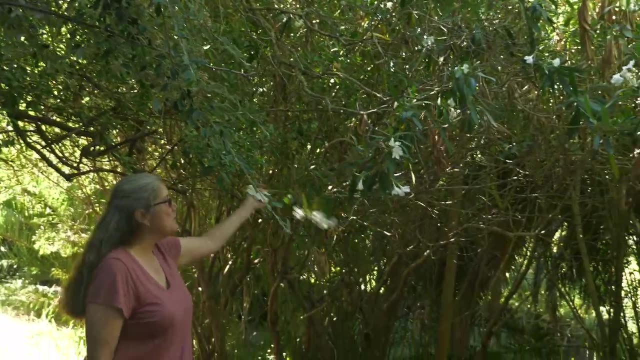 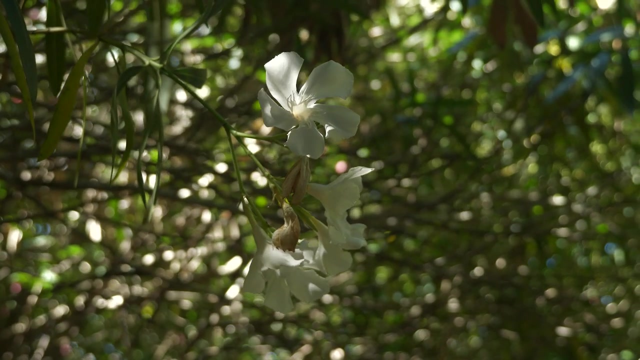 store in a paper bag You can distribute in desired locations in the fall or trade seeds with friends. That's it. Removing plants with little ecological benefit but that create a fire risk can create opportunity. Oleanders not native to North America provide little ecological. 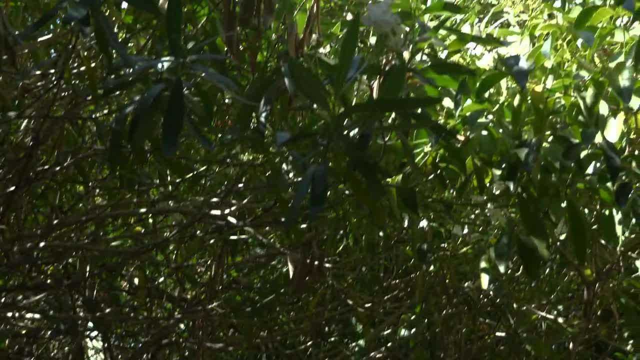 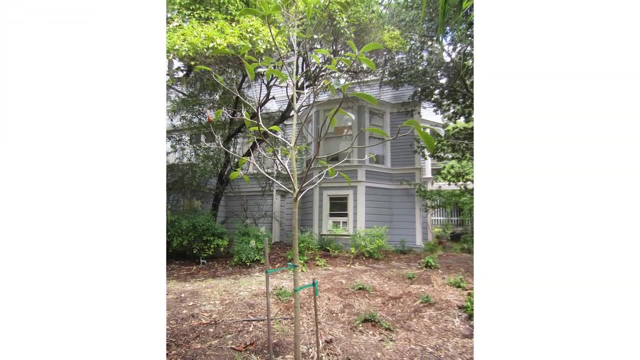 benefit to native species. In addition, the hedge laddered between the front privet hedge and the home- In this case a loquat tree- was transplanted from a bed next to the house and was placed where an oleander hedge was removed. The loquat tree provides pollen and 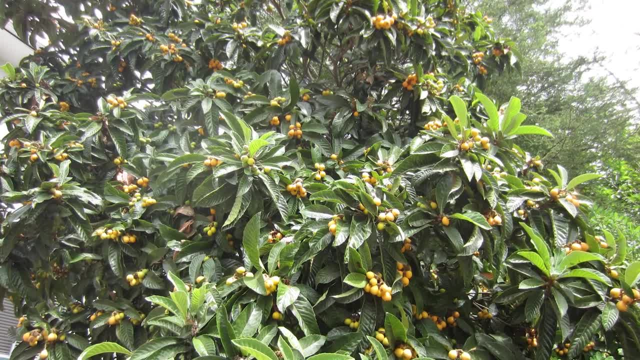 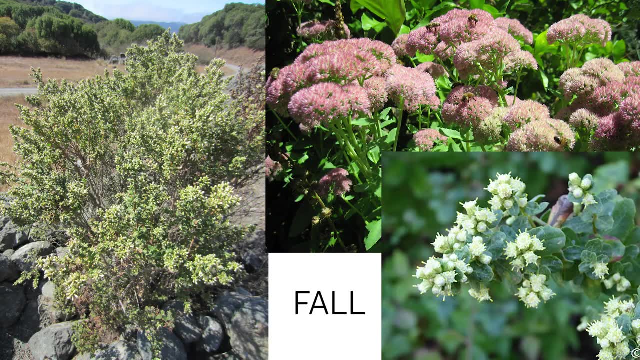 nectar for pollinators in late fall and fruit in the spring, but it's not good for the in the spring. Try to select a variety of plants that provide pollen and nectar during different times of the year. To maximize the benefits to pollinators, it's often best to plant the 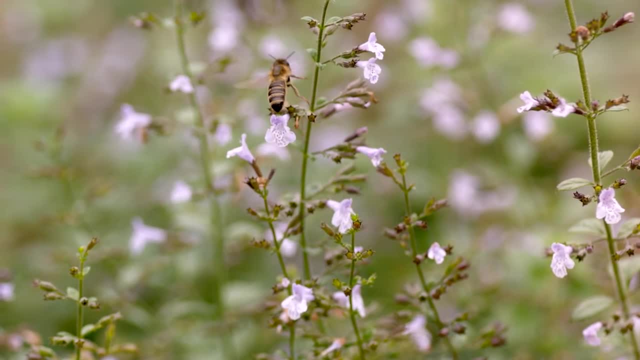 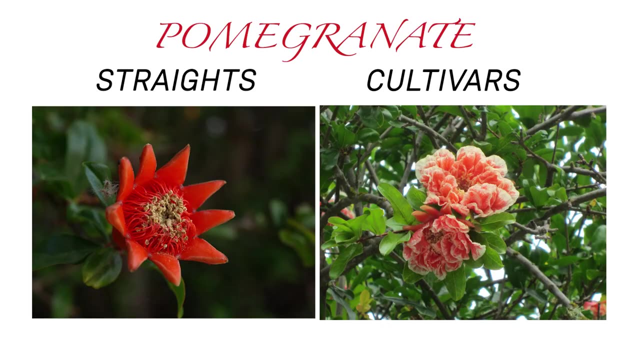 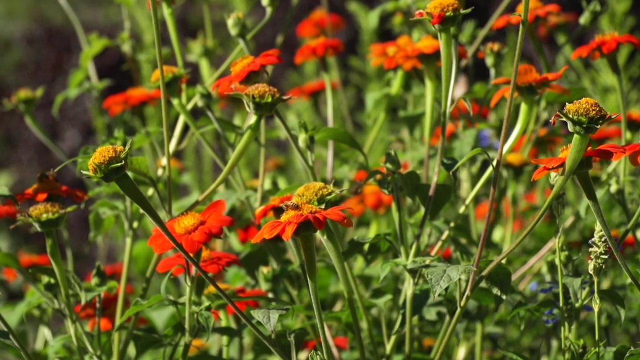 straight species as opposed to cultivars. Many cultivars have been selected and bred for aesthetics, but would be unable to reproduce without human assistance because their pollen and nectar is unavailable to pollinators. If you need help, just observe which plants you see the bees visiting. 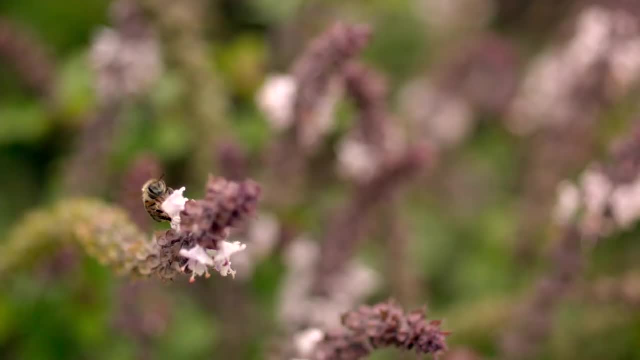 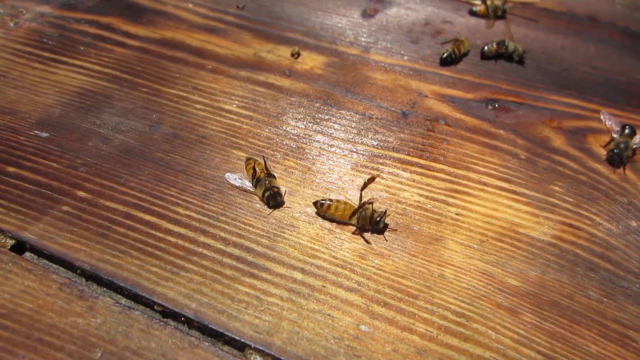 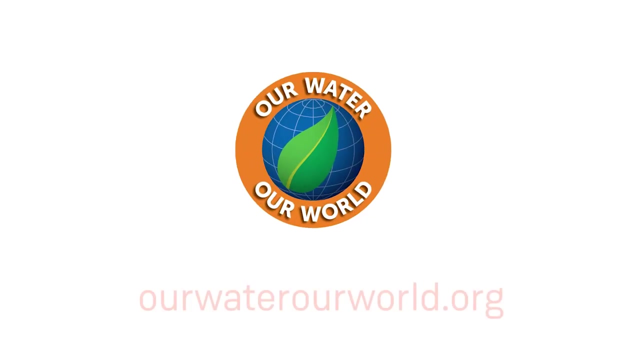 They'll let you know what they prefer. A final comment: One of the easiest ways you can protect pollinators is to eliminate chemical use in the garden. A pesticide is a pesticide and you may be harming beneficial insects as well as polluting our waterways. For advice on less toxic alternatives. 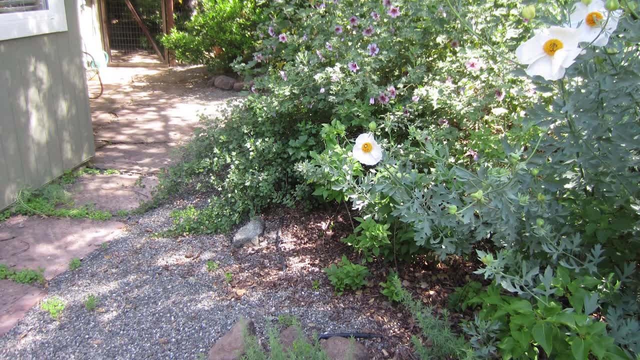 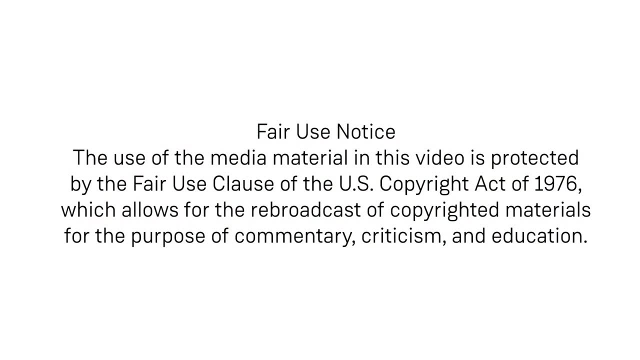 reach out to Our Water, Our World. Fire Safety can be both beautiful and support biodiversity. We can have it all with careful planning. 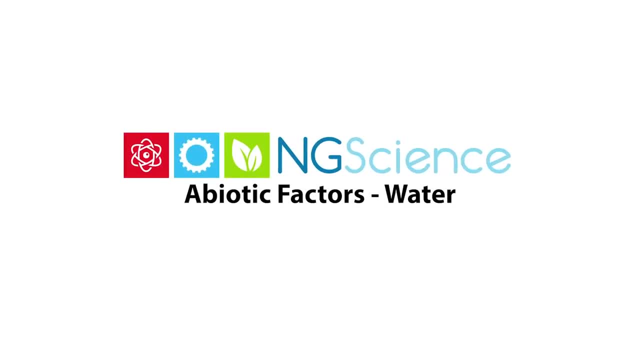 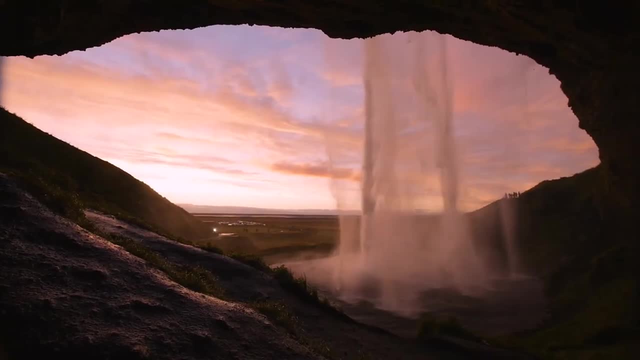 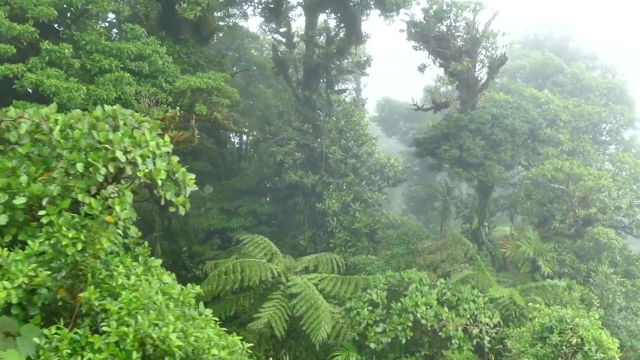 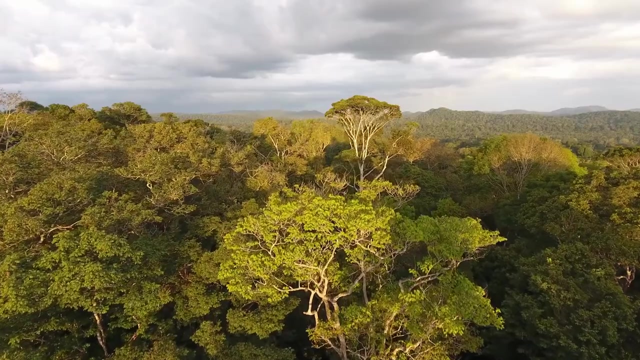 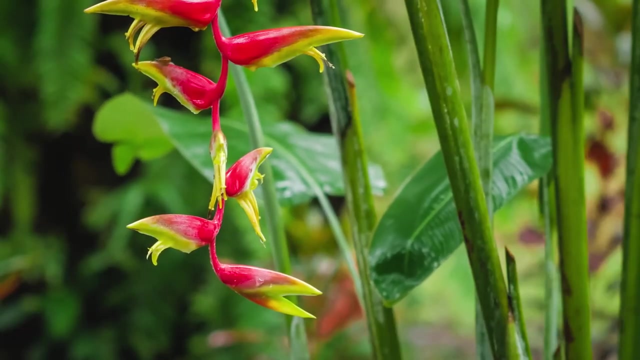 Water is essential to all life on Earth. The availability of clean, fresh water has a large influence on the components of an ecosystem. Plants need water to make food. during photosynthesis, Plants also use water to transport food and minerals to all parts of the plant.